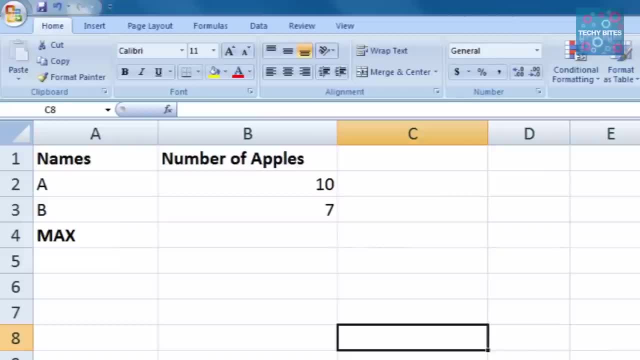 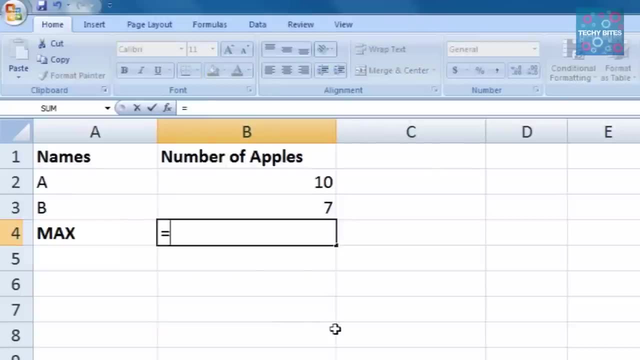 If we had to determine who had more apples, we could simply use the maximum function To write this function. just click on the cell where the desired output is to be displayed and write the function as follows: Define the max keyword, then open the round bracket. 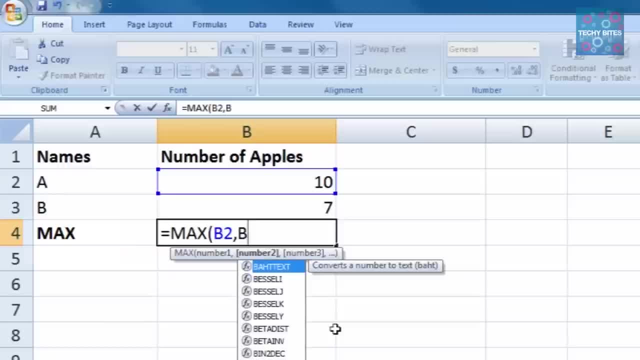 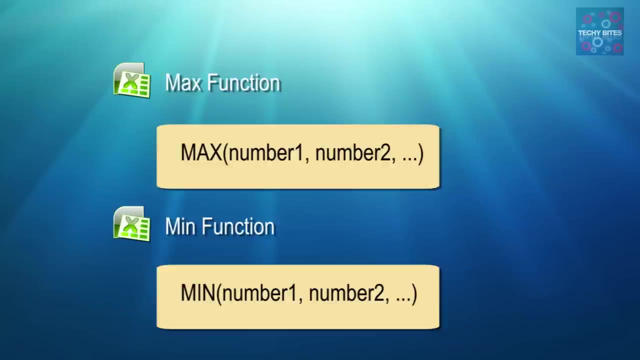 type in the two cell values b2 comma b3, and then close the round bracket. It's simply as: max parentheses b2 comma b3, close parentheses. Now for minimum functions. let's consider the following example. Let's say a, b and c are three kids who have some set of flowers with them. 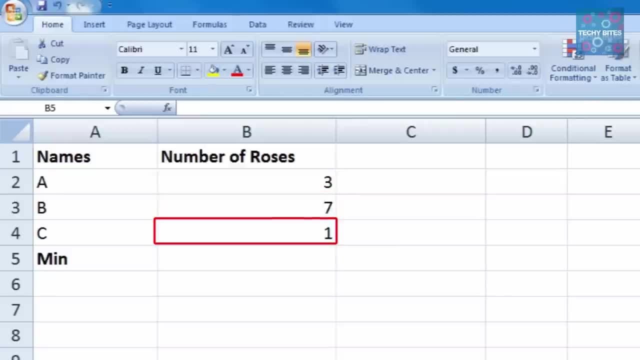 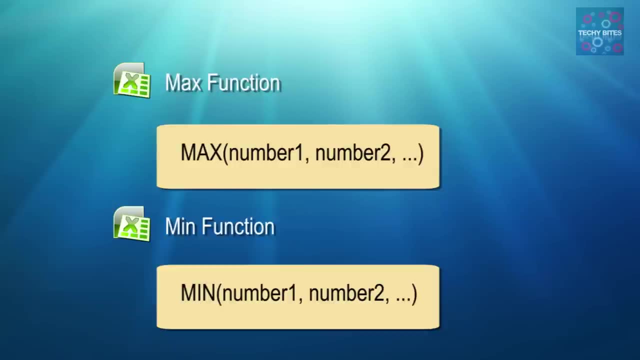 a has three roses, b has seven roses and c has one rose. Now to determine who has the least number of roses, we use the minimum function. The function for this example is defined as follows: Define the min keyword, then open the round bracket. 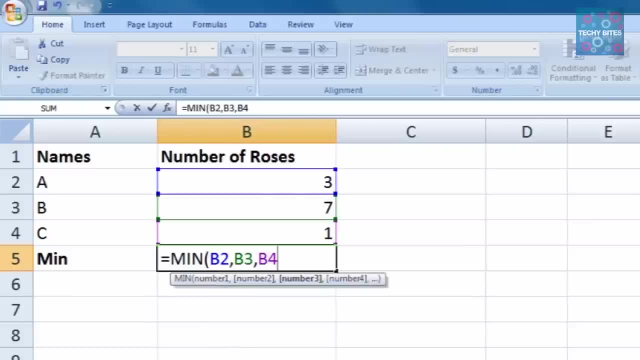 type in the three cell values b2,, b3, and b4, and then close the round bracket. It's simply min b2 comma b3, comma, b4.. Now let's do one more example. Let's say we purchased a list of items at the supermarket. 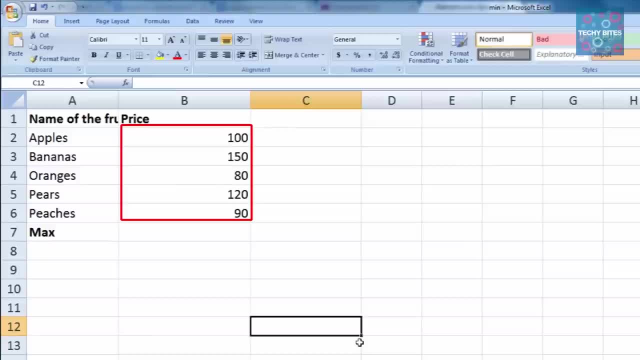 and we want to determine the item that's the most expensive amongst the list of items we've bought. So it would be easy to use the max function. The list of items is written under column a and their prices in column b, as follows: 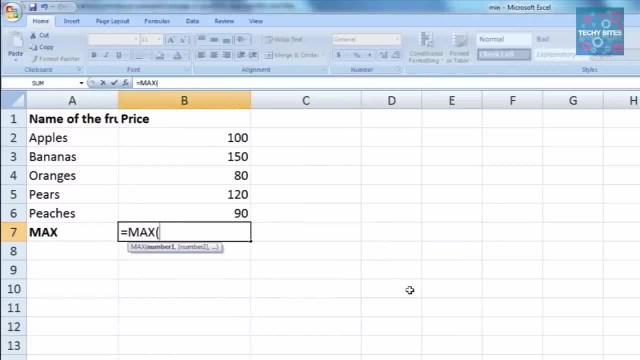 The formula can be written as: max- open round bracket, then type in the cell names followed by the comma operator and then close the round bracket. It can be written as max- b2 comma, b3 comma, b4 comma, b5 comma, b6. close parentheses or simply max. open parentheses. b2, colon, b2,. 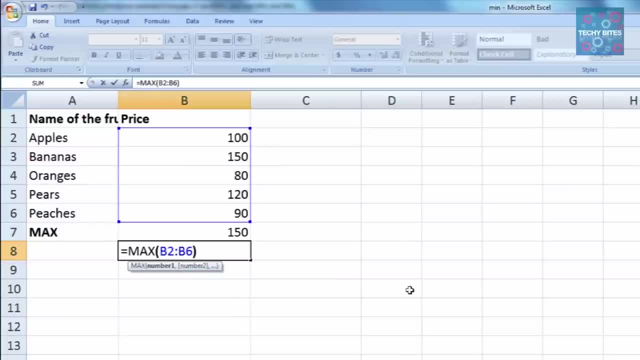 and then close the round bracket. The column signifies that the rows within the specified range are included. Likewise, to determine the least expensive item in the list, we can use the minimum function. So for this example again, the function would be written as min parentheses: b2 comma. b3 comma, b4.